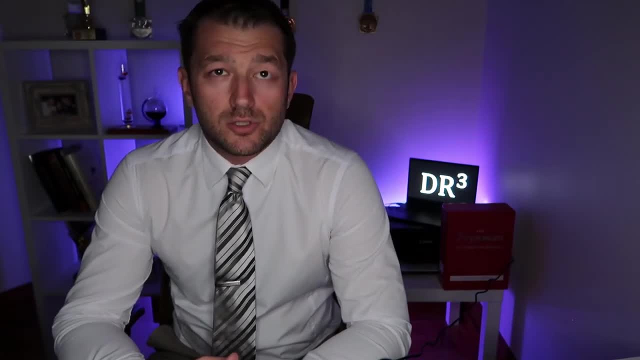 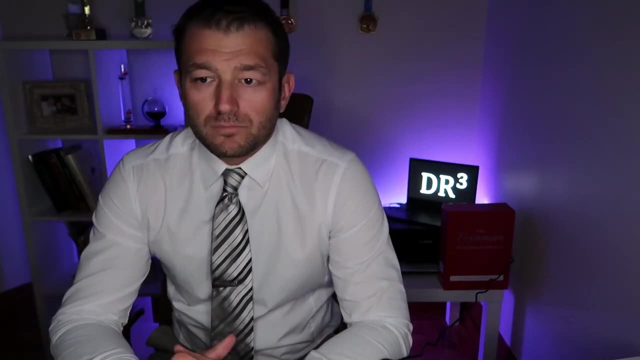 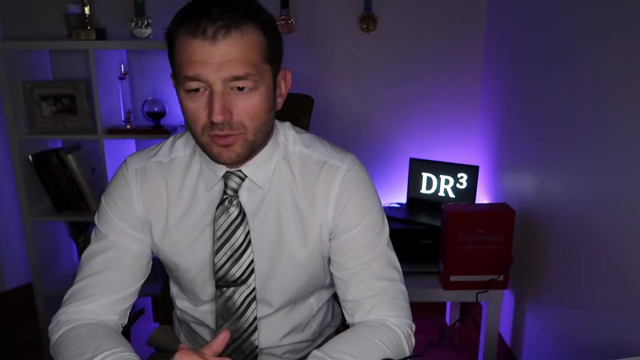 for the wind turbine blades rotating. it is also responsible for the warm air that comes out of the oven- hot oven- when you open it and, in fact, it is also responsible for you being able to breathe and listen to this video. At the end of this video, you will be able to understand how the breathing of 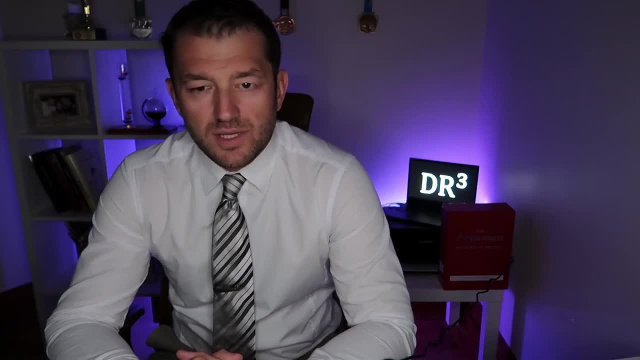 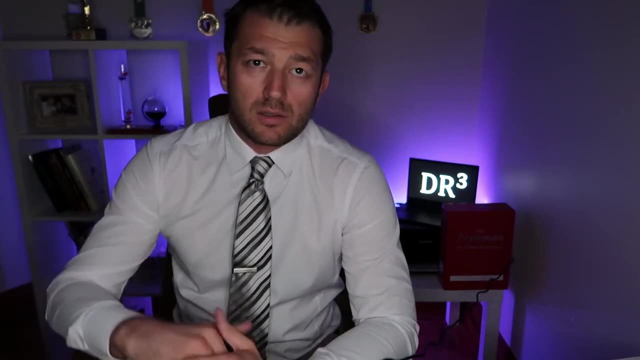 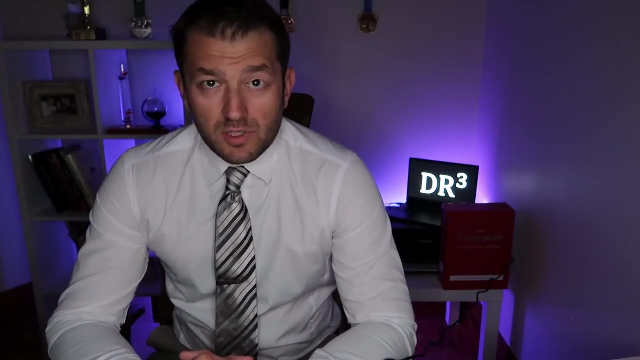 a human being works thanks to the pressure gradient force, and the subject of wind turbine blades rotating due to the pressure gradient force will be in another video In our wind energy series. So, in very simple words, qualitatively, the pressure gradient force. 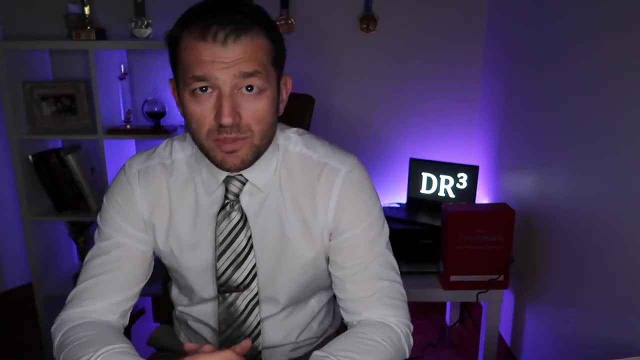 arises due to the differences in pressure between two points in the atmosphere. The higher the pressure difference, the stronger the force, And the pressure difference usually arises due to the differences in temperature and so on. But for this video we will just say there is a pressure. 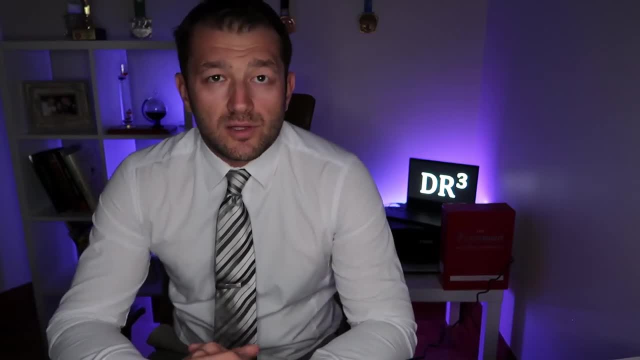 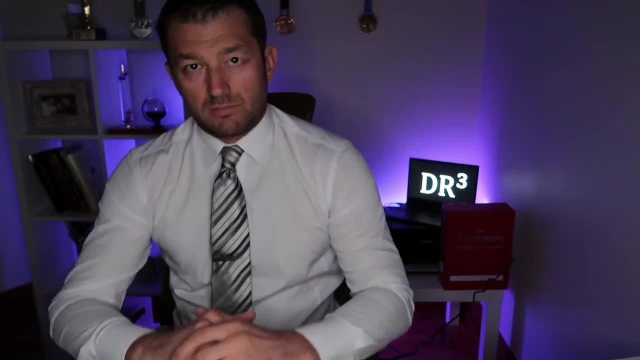 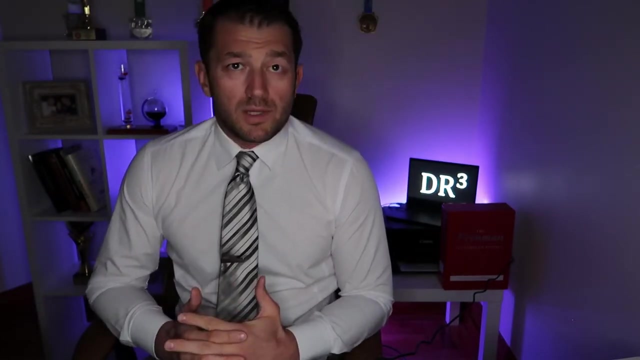 difference for some reason, and that causes the pressure gradient force, And due to the pressure gradient force, air tends to move from the region of high pressure towards the region of low pressure. So this is pretty much all that we can say qualitatively. 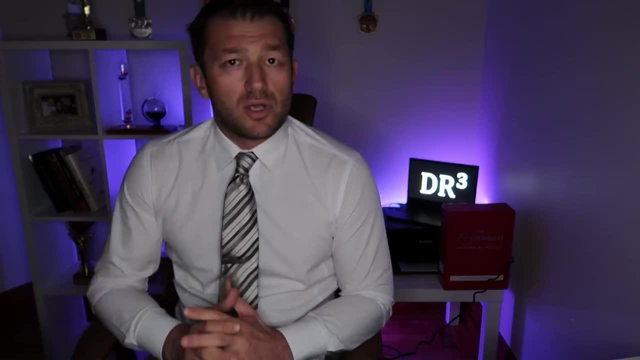 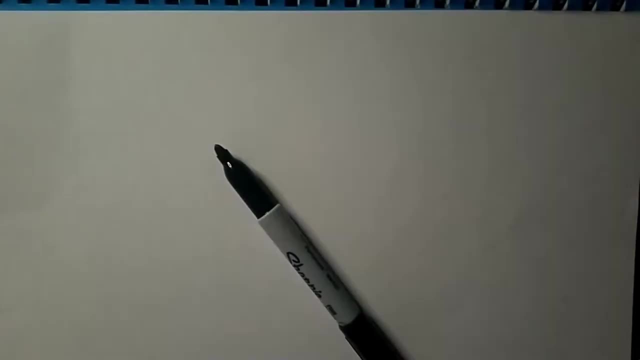 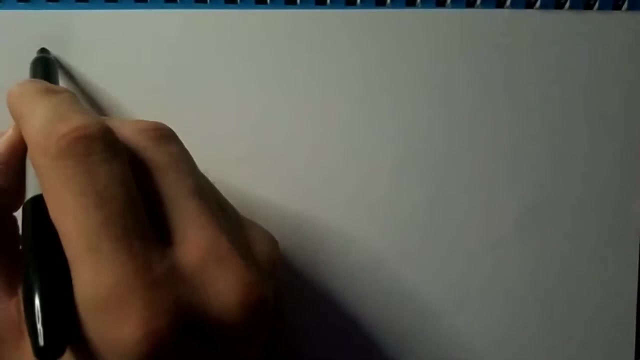 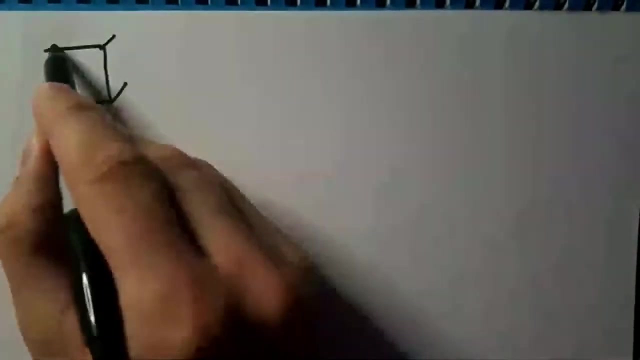 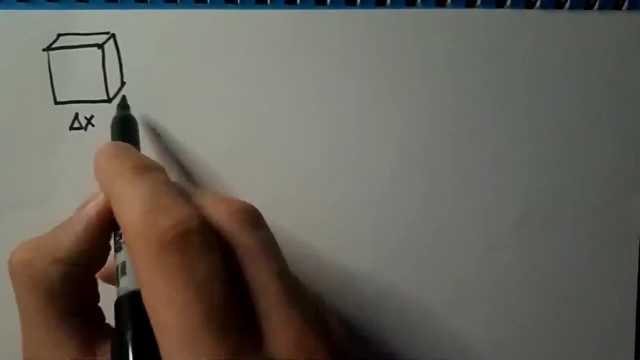 about the pressure gradient force. So now let's go and try to derive the mathematical form of this extremely important force in our everyday life. To do so, I will consider a cube of air like this one, for example, that has sides- delta x, delta y, delta z. So this is a three-dimensional object, clearly. 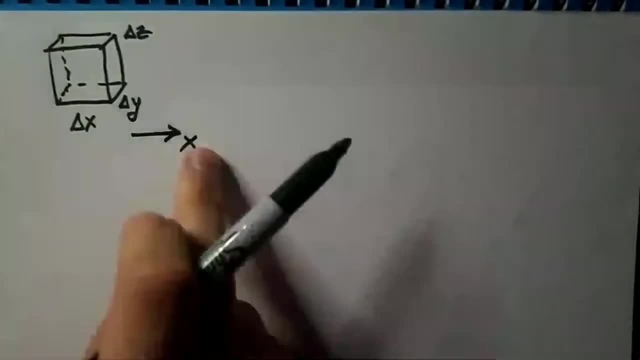 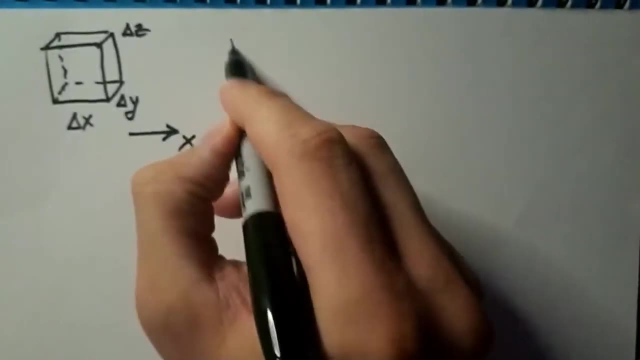 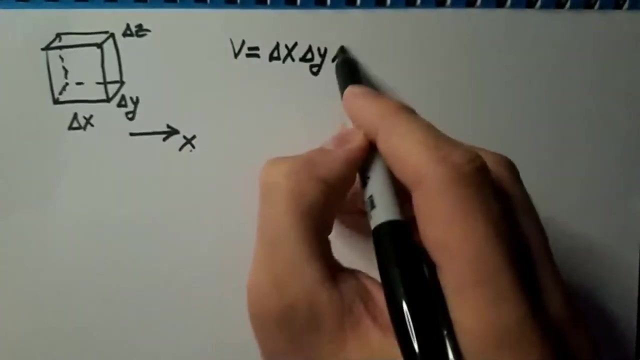 I will say: this is my x-axis and this is the. the x-axis, The square of this square is the vertical therapist. It has difficulty in terms of peaks because it's equal to the vectors of the working слов. It has difficulties in terms of distribution of the Osaka to the 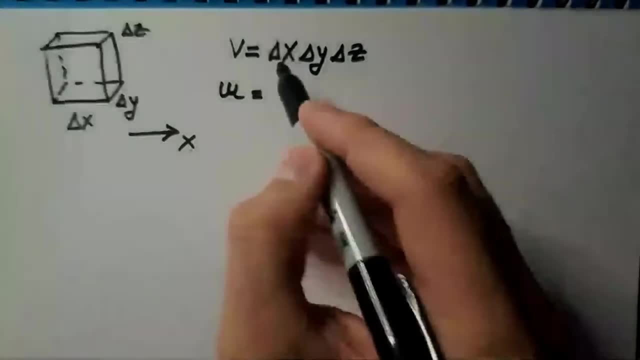 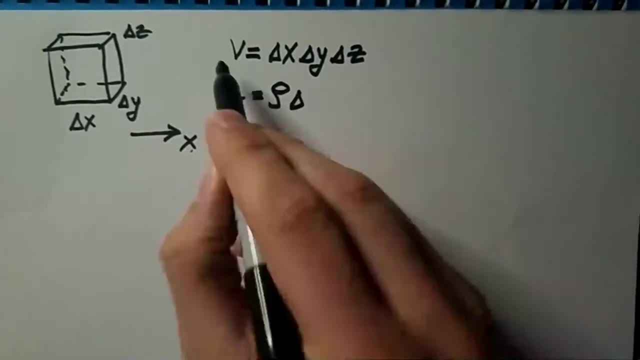 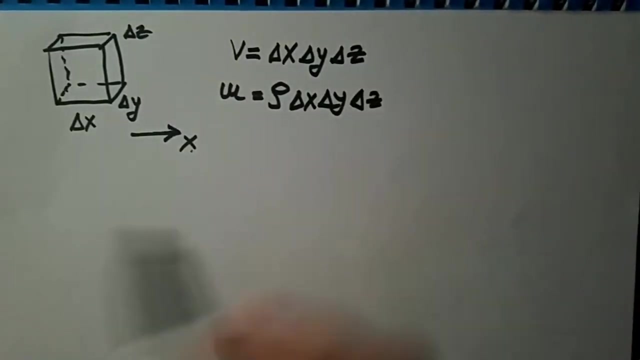 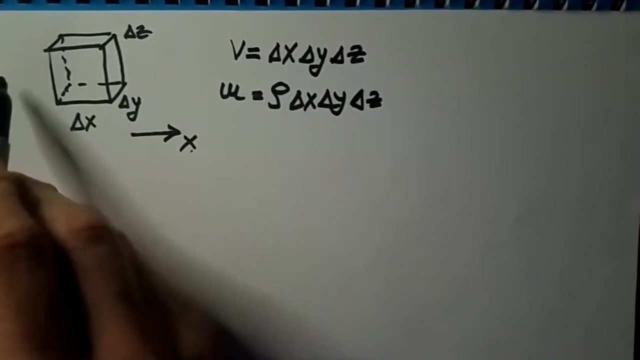 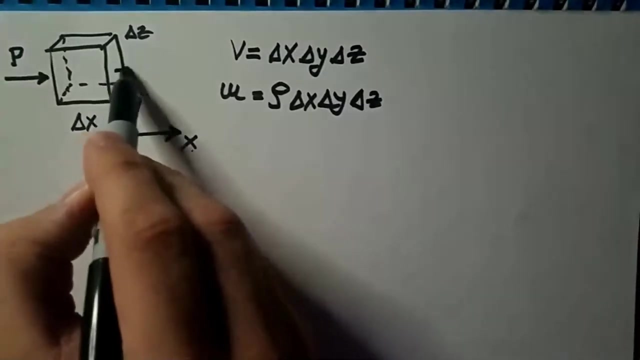 givenmil and its properties. but this value isений clearly the enh value of the restricted f or the level or weight of the x delta, y, delta z. Okay, now let's consider that in the x direction there is a pressure P on this side of the box and there is some other pressure P plus. 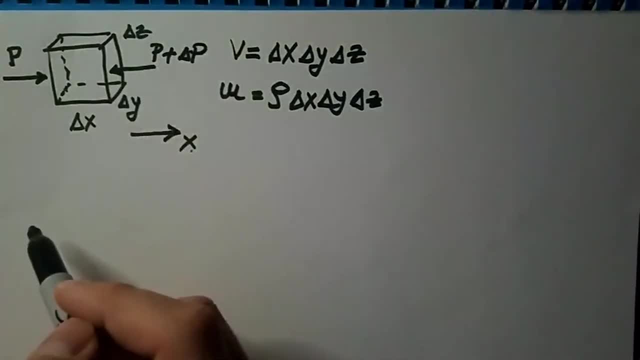 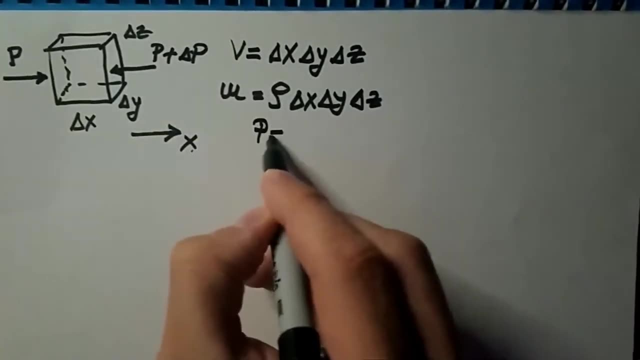 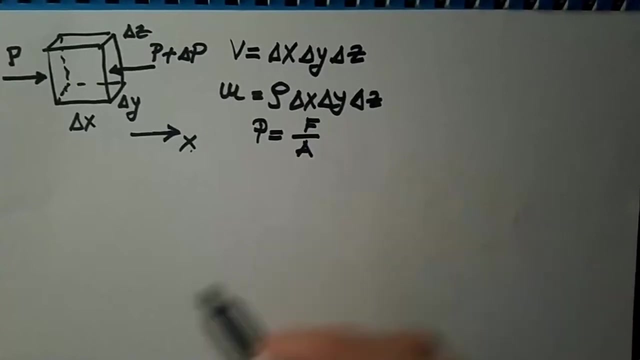 delta P on the other side of the box. We know also that pressure is force per area. Okay, now, when we know all that, let's write down the second Newton's law in the x direction. The second Newton's law in the x direction says that mass 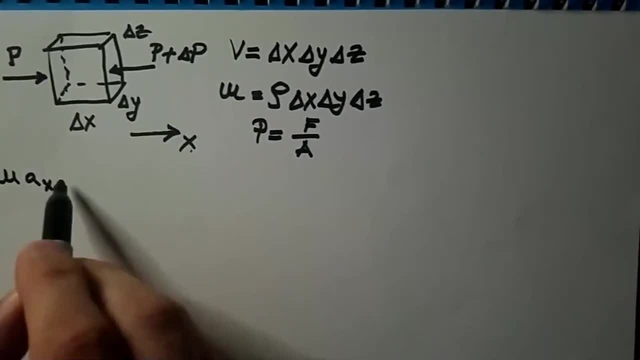 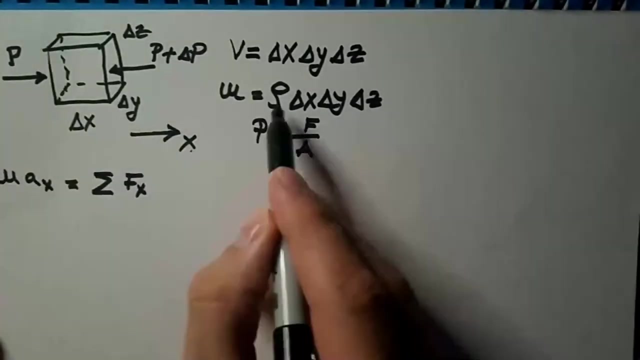 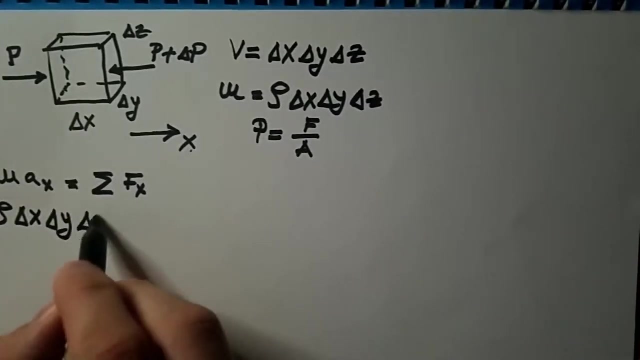 times acceleration in the x direction is the sum of all forces in the x direction. Well, now we just need to plug in everything in this equation and we will get that. mass is this density times volume, which is dx, dy, dz times acceleration in the X direction is the sum of all forces. 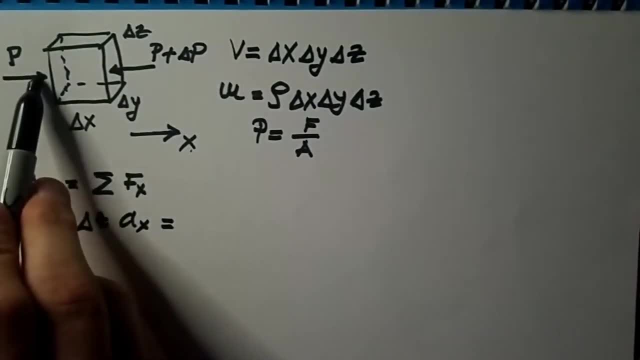 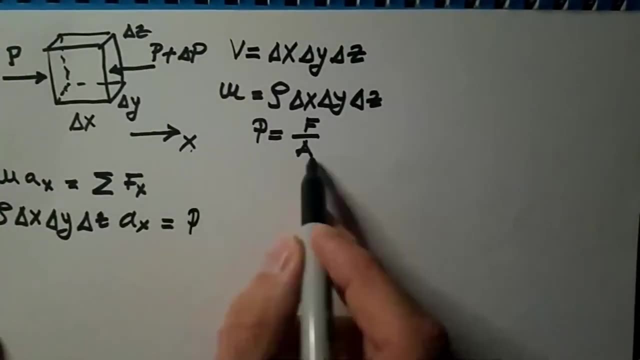 Well, have force here due to pressure, and the force is pressure times area. so, pressure times area, what is the area of this side? well, clearly, it is Delta Y, Delta Z, and then I have force in the opposite direction, in the negative direction of x-axis, so minus, and this force is P plus Delta P, and again, area of this side. and 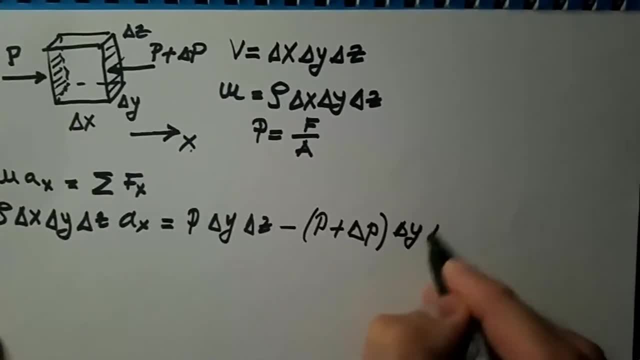 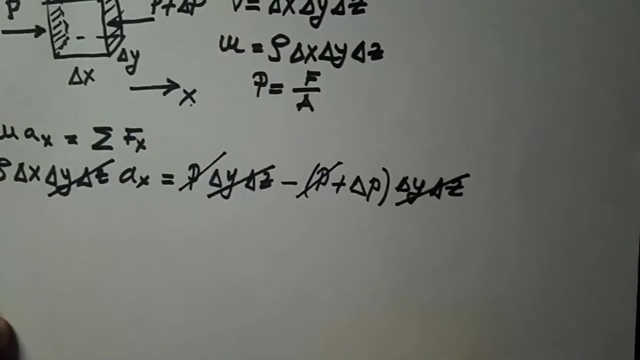 the area of this side is the same: Delta Y, Delta Z. now we can cancel Delta Y, Delta Z, Delta Y, Delta Z and Delta Y, Delta Z here, and in fact we can also cancel this P, P plus P and minus P, and then we end up with a rho, which is density. Delta X, A X. 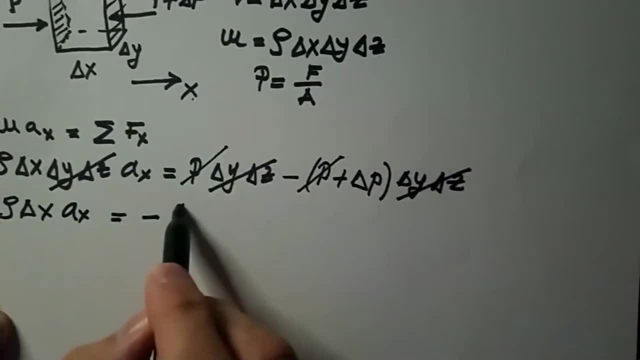 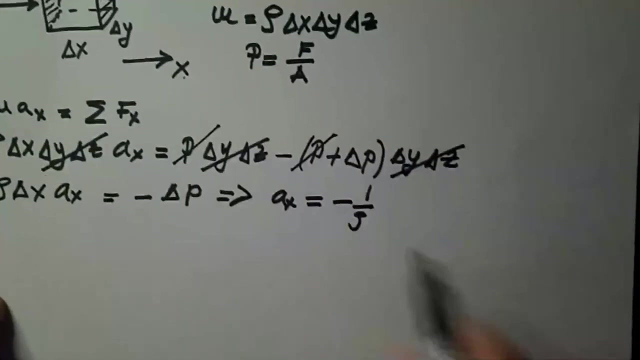 is equal minus Delta P, or I can rewrite this as A X equals minus. I will move rho to the other side, one over rho, delta P over Delta X, and this is the acceleration due to the pressure gradient force, or pressure gradient force per unit mass. now I would like you: 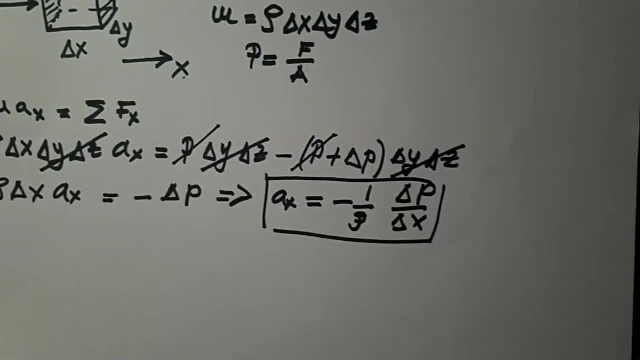 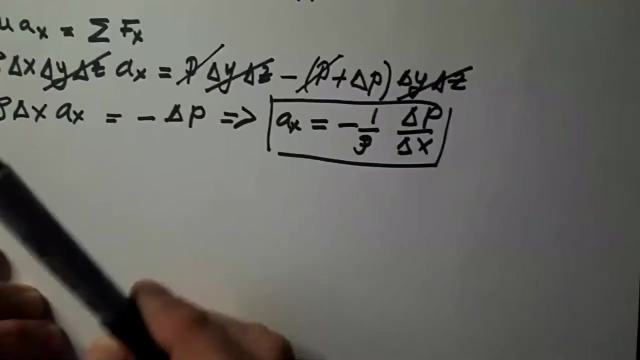 to understand that when we are using pressure, gradient force in everyday life, which are finite differences, then we always use it in this form of where we we have a finite difference of pressure and some finite distance. again, thanks to our old friend Isaac Newton, we can put this in a form of infinite. 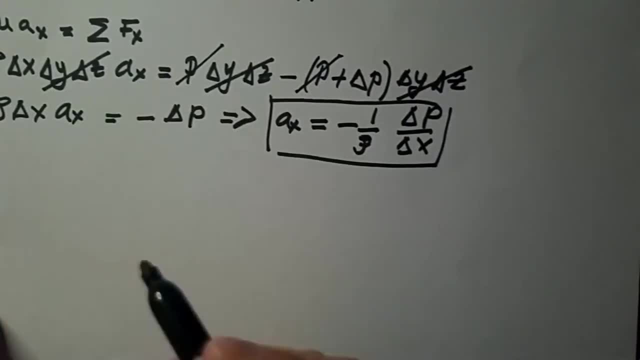 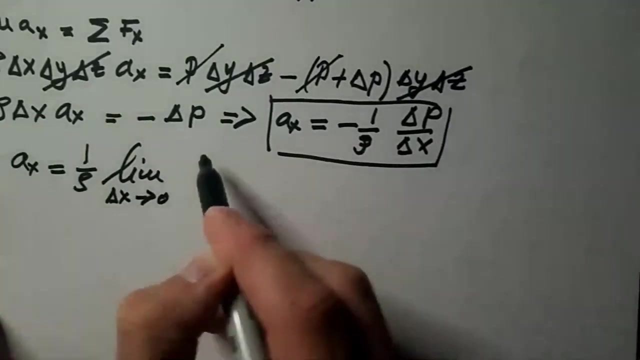 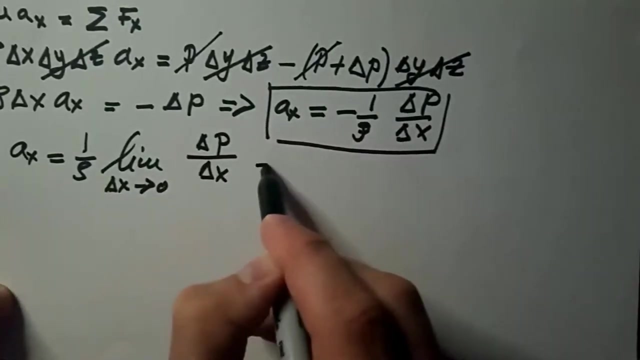 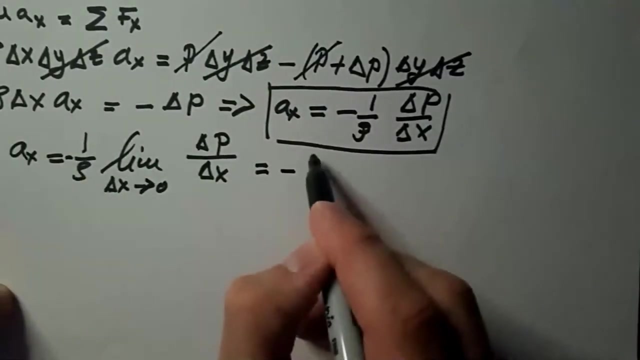 similarly small distances, and I always have a problem saying that word in other ways. I can say: A X is 1 over rho limit when Delta X goes to zero. delta p over delta x, and then i hope you know enough calculus to realize this is part. there is minus here, this is partial derivative, minus one over rho, delta p over delta x and this: 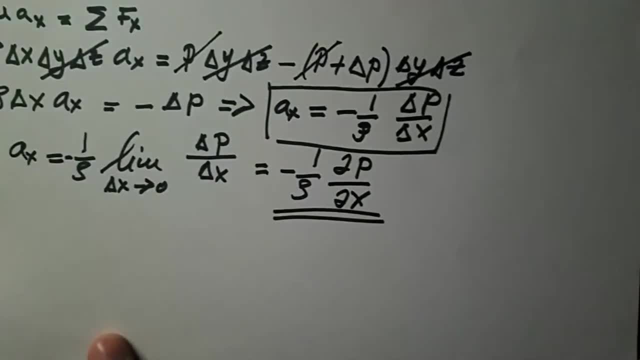 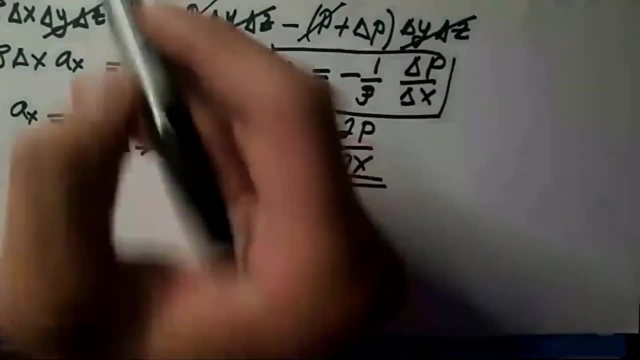 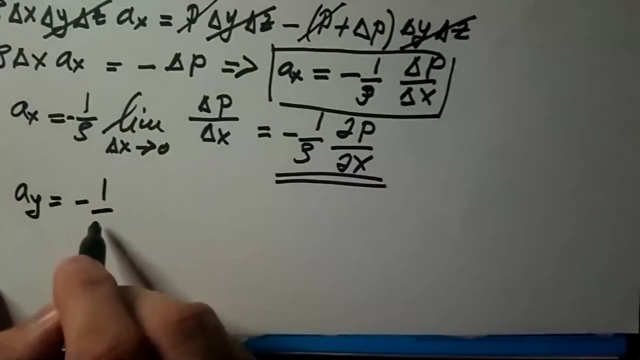 is the pressure gradient force in a, you know, in a mathematical way, expressed in infinitesimally small differences. clearly, i can do the same derivation for the other two direction and then i would get: dy is minus one over rho, delta p over delta y and a in the z direction or acceleration. 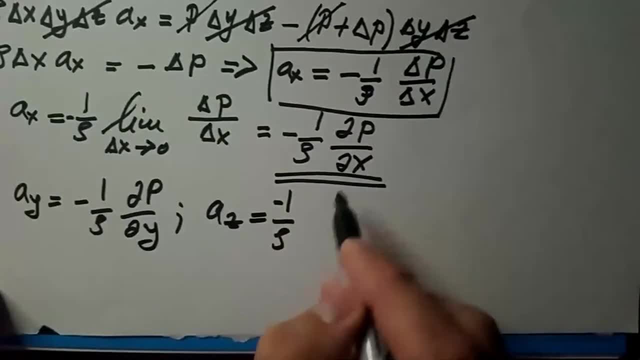 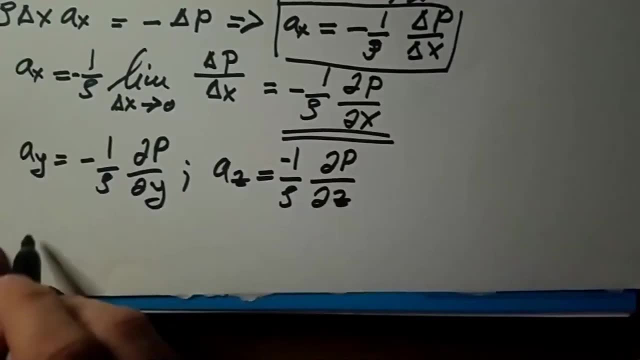 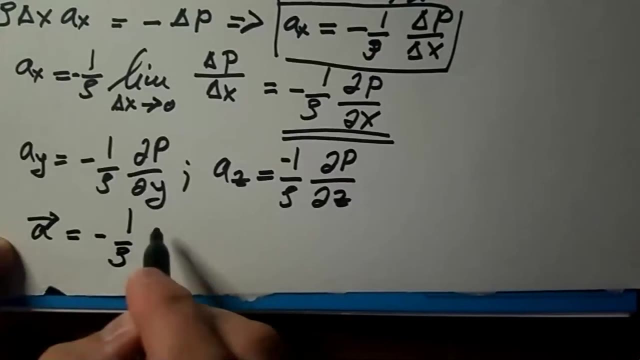 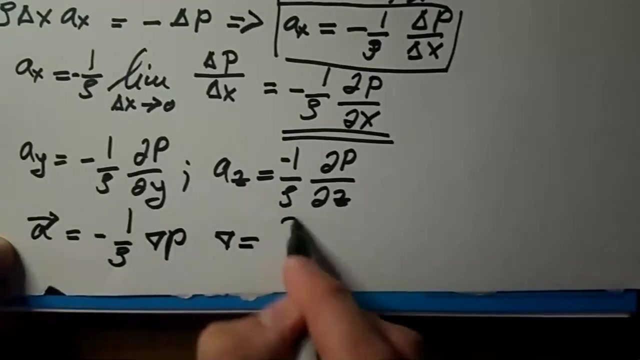 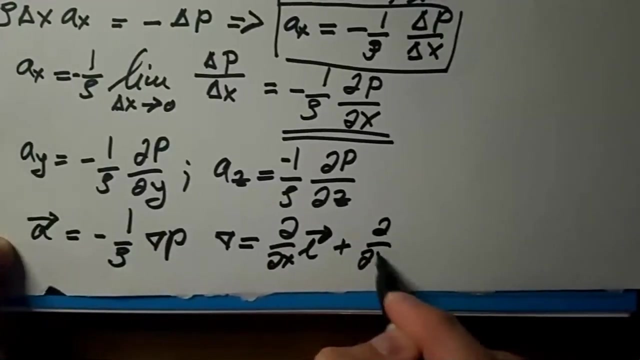 in the z direction, minus one over rho, delta p over delta z. another way we sometimes put this is we say that acceleration due to pressure gradient force in a vector form is minus one over rho, nabla p, where nabla is a differential operator. delta, delta x, i plus delta, delta y, j and plus. 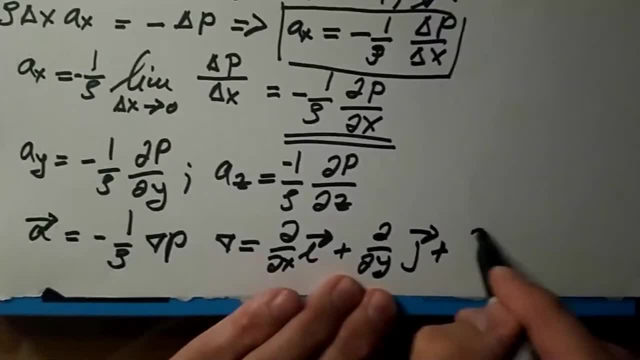 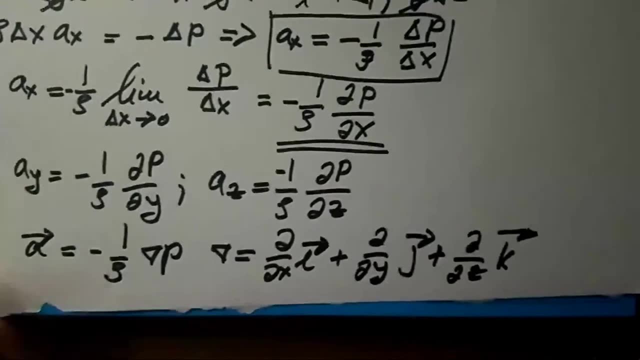 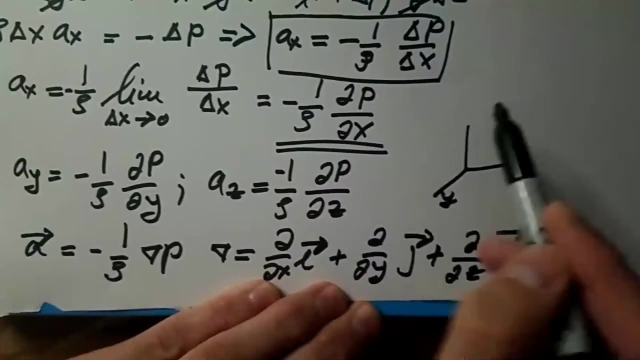 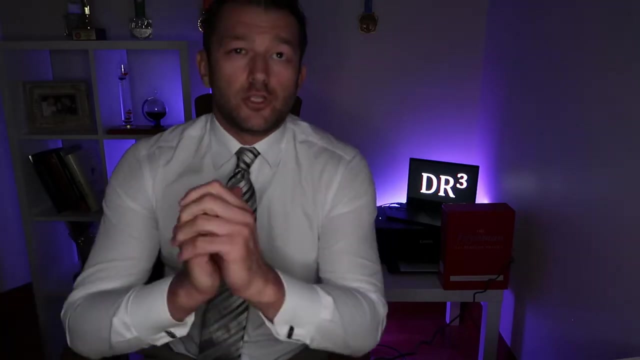 delta, delta z k, where i, j and k are the unit vectors in the x, y and z direction. so if this was my y direction is if this was my x direction and z coordinator direction, then these are the unit vectors: i, j, k respectively in these two directions. so now you understand the. 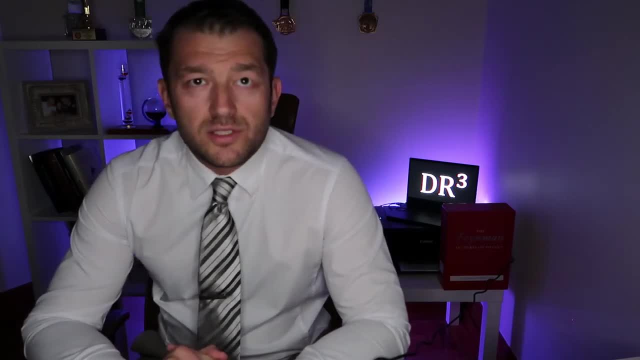 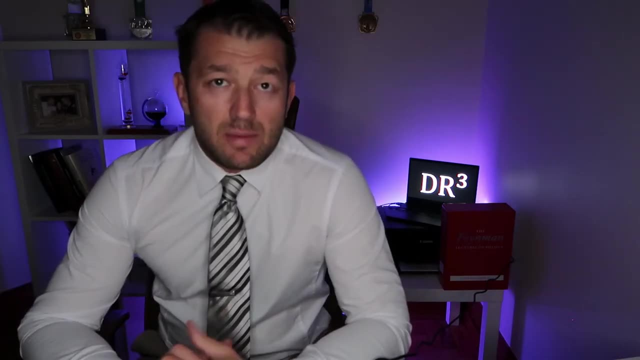 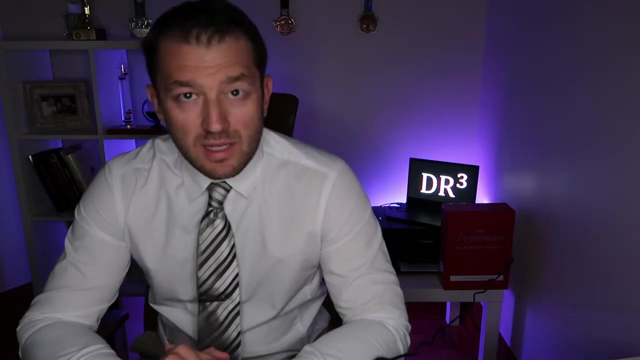 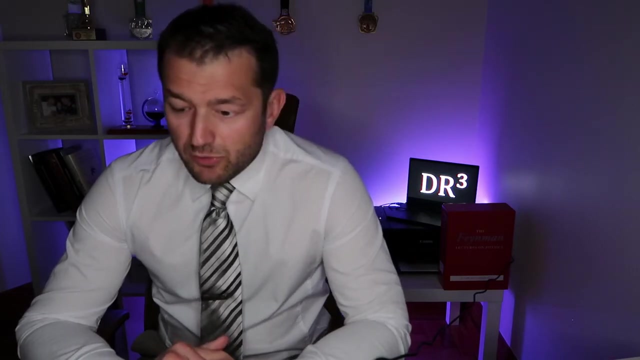 vertical form of the pressure gradient force. now let's use this to this derivation and these equations to examine some of the phenomena in the real atmosphere. in the real atmosphere, we use this expression, for example, to analyze synoptic pressure charts or synoptic pressure maps, where we can indeed estimate the pressure difference and the pressure gradient. rather, 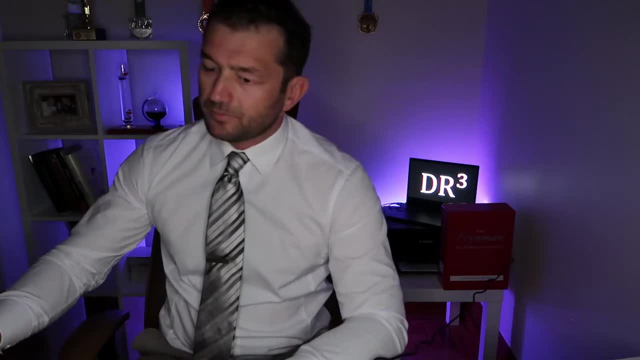 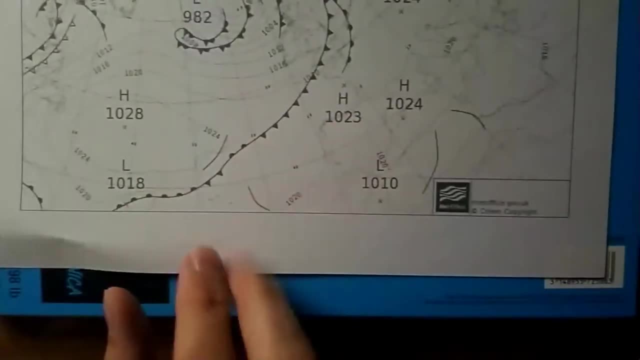 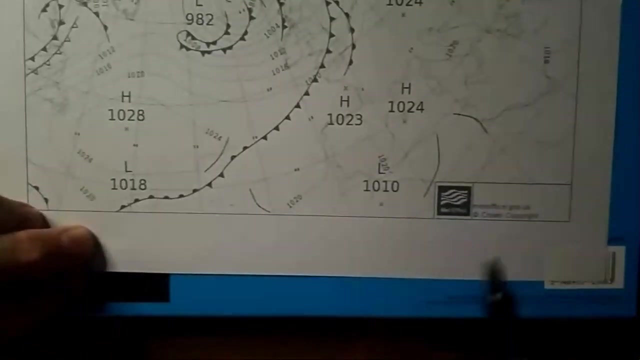 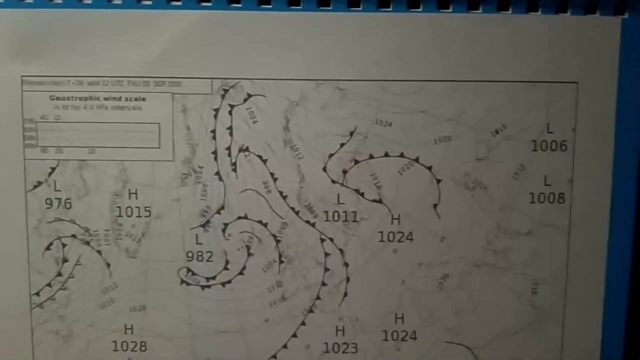 between different points above earth's surface. so here i printed a surface pressure map from a met office, so i let me just adjust. so this is the surface pressure map from met office for uh today and uh, what we see here is a bunch of lines. the lines that are important for us are these full. 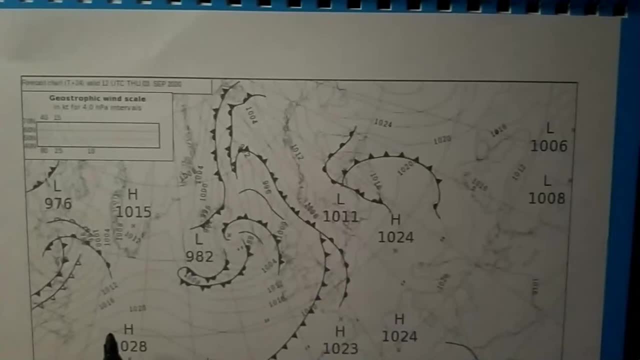 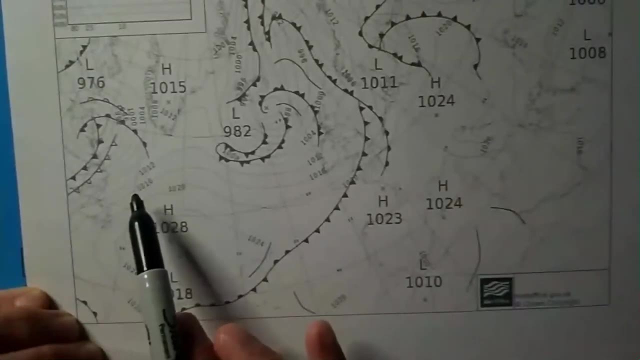 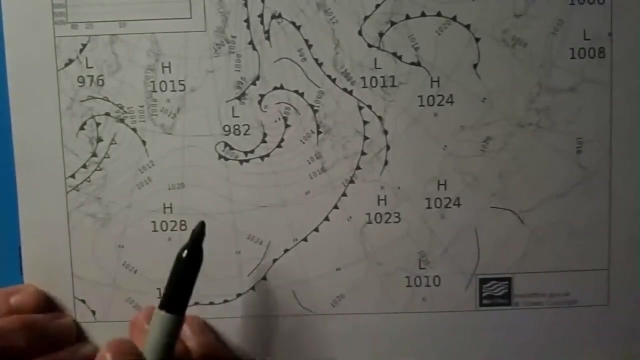 lines that i hope you can see that show surface pressure in millibars. so we have 16 millibar, we have six hundred uh 1016, 1020, 1024 millibars. so let's use now the uh, this pressure map, to estimate. 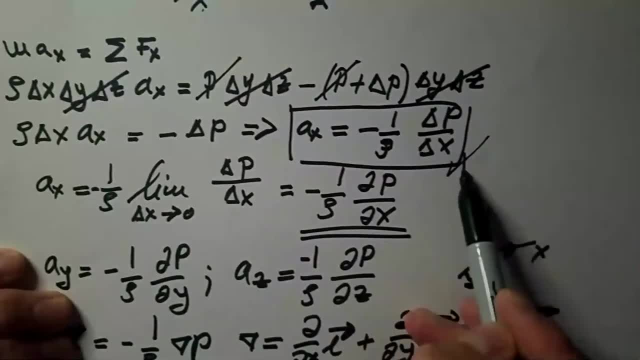 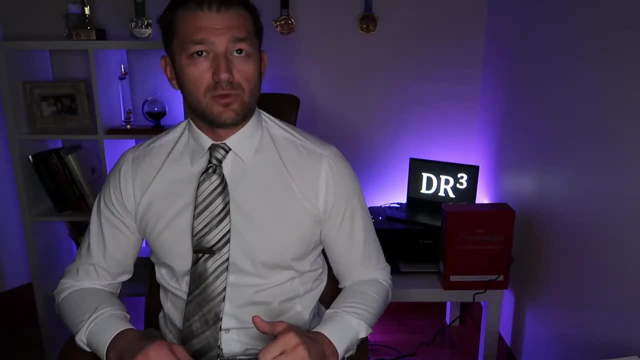 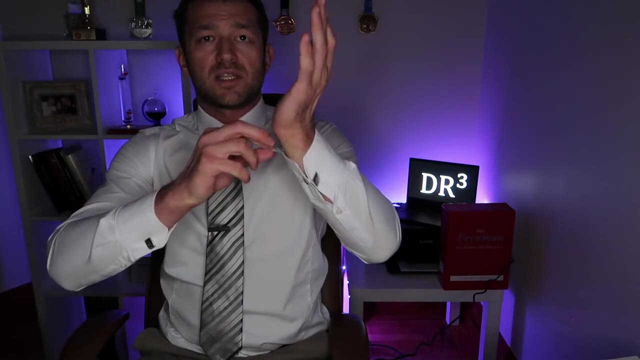 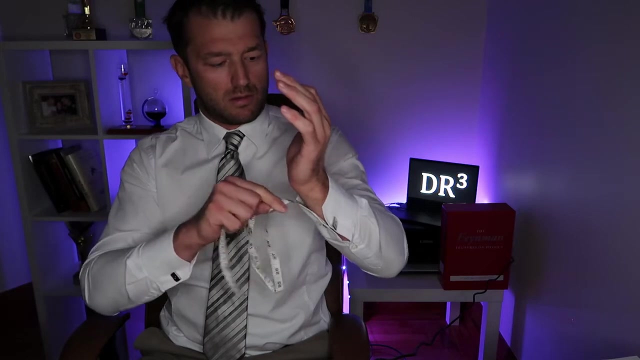 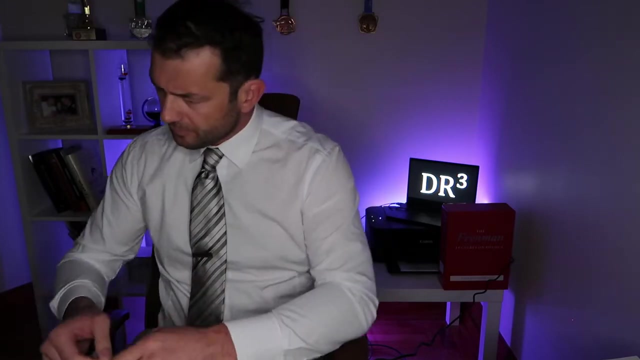 the pressure gradient in this form here right now to do that to? to do that i would need some ruler that that will help me to measure the distances, and it just happened that i have a meter tape here here. who would expect that? so let's say we want to estimate the 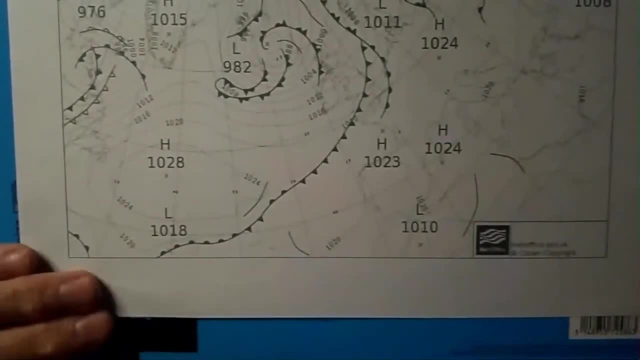 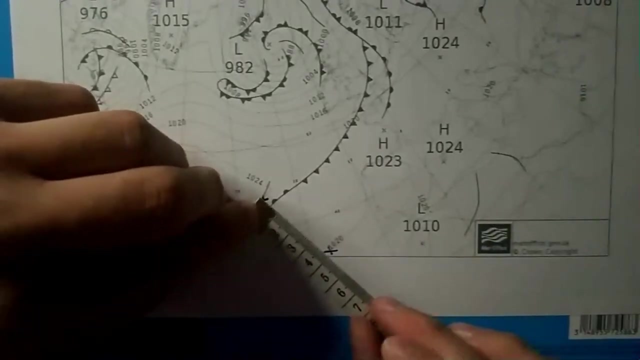 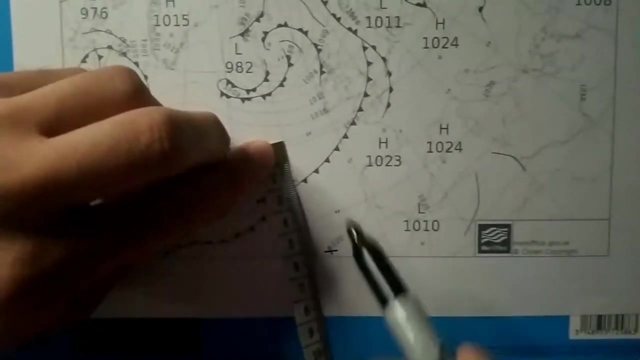 pressure gradient, uh, between, let us say, between, this point here and this point over here. okay, now, if I use this meter, this ruler, the distance is about 4 centimeters. but I can also see that the distance is about 4 centimeters between this latitude and this latitude and and this latitude, and I know the distance between. 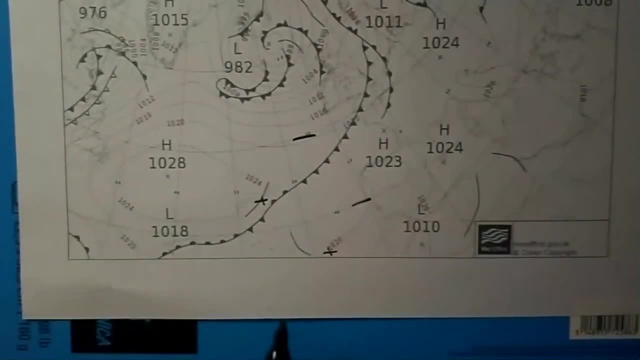 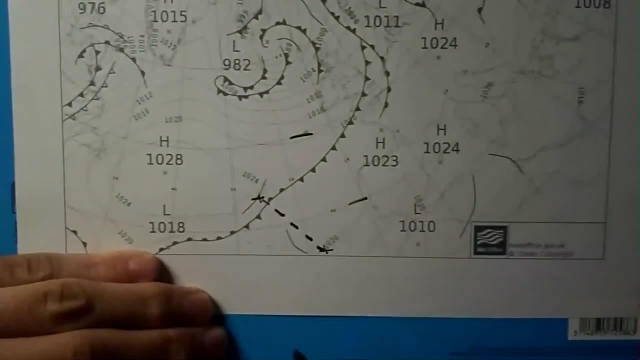 latitudes is about 111 kilometers. so I can say, if I take this distance, that, in this particular case, Delta P over this distance, Delta n, let's call it- is equal. well, Delta P: this is 1024, this is 1020, so it is 4. 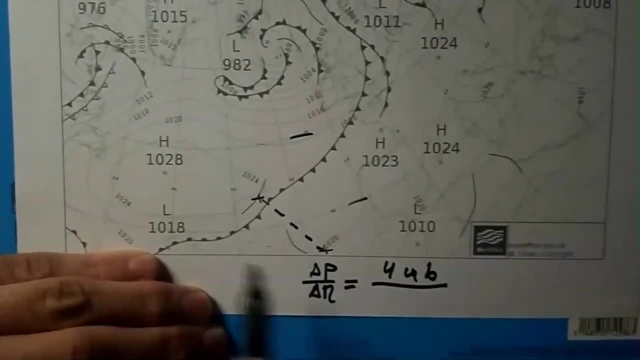 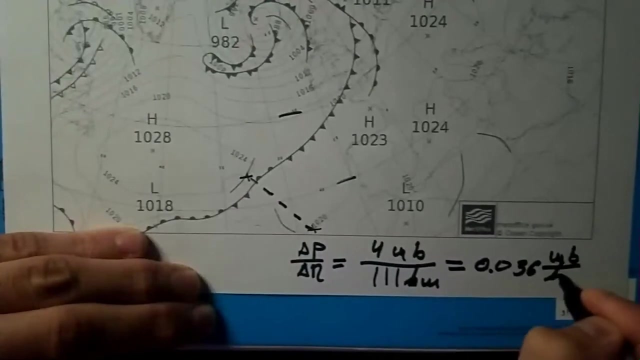 millibars divided by 111 kilometers approximately, because I know this distance is the same as distance between latitude circles, and this, this and the distance between latitude circles is around 111 kilometers. so if I do this, I should get. if I divide this, I should get 0.036 millibars per kilometer. 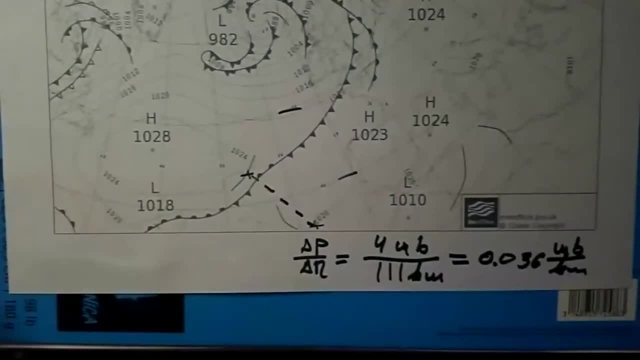 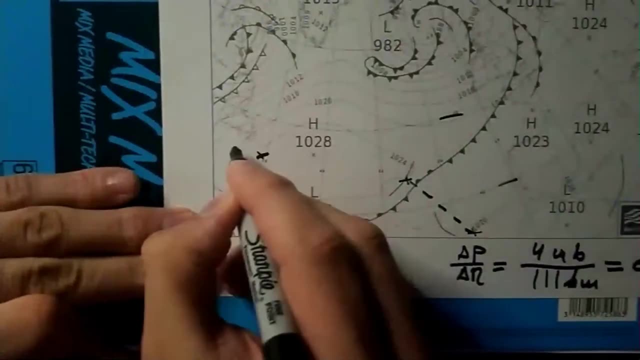 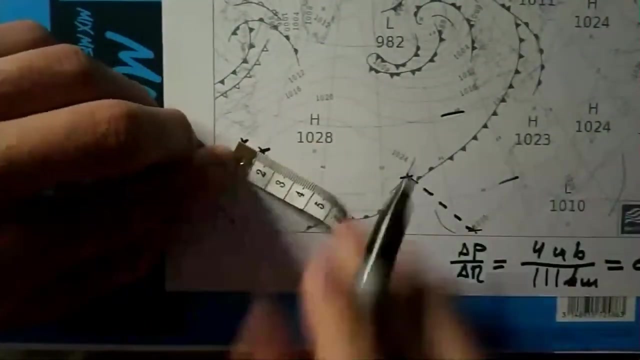 Now let's do the same exercise, but for example, for these two points- I'll take this point here and this point here- The distance here is, as you can see, around one centimeter. Here was four centimeters, here is one centimeter, so that is four. 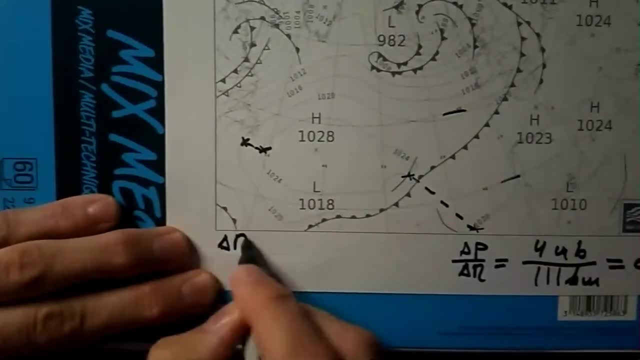 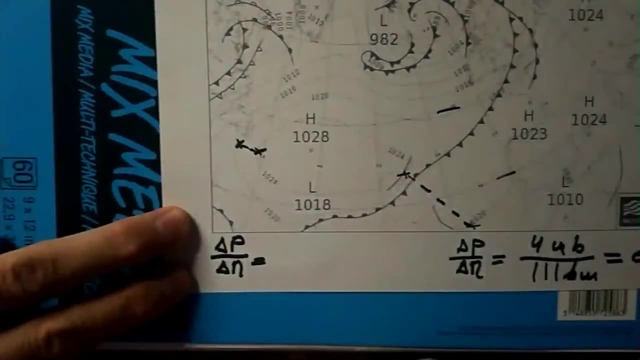 times smaller. So here delta P over delta N is the same 4 millibars. but over the distance of 111 divided by 4 is around 28 kilometers, so I get it is 0.143 millibars per kilometer. What we can conclude? that the pressure gradient here is about four times the. 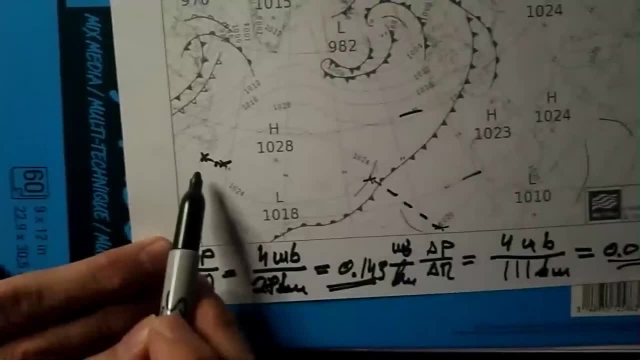 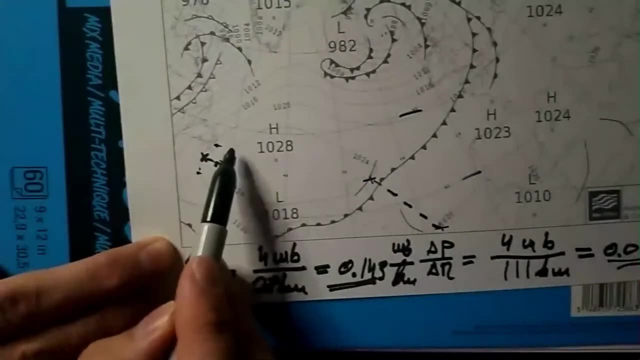 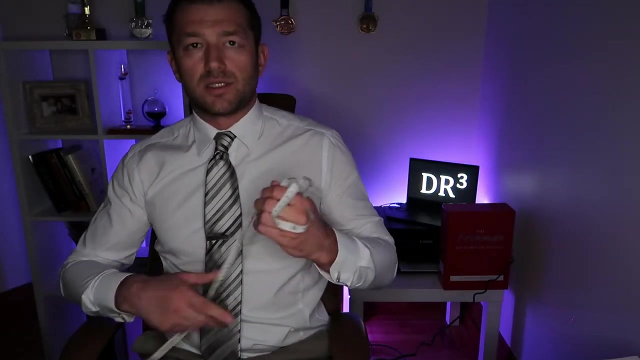 pressure gradient here and you can see that by the distance between isobars- Isobars are the lines of constant pressure- You can see that isobars are much closer here compared to here. So what we concluded from this analysis is: if we have 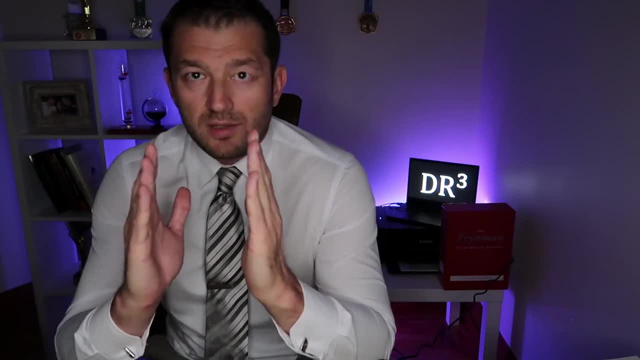 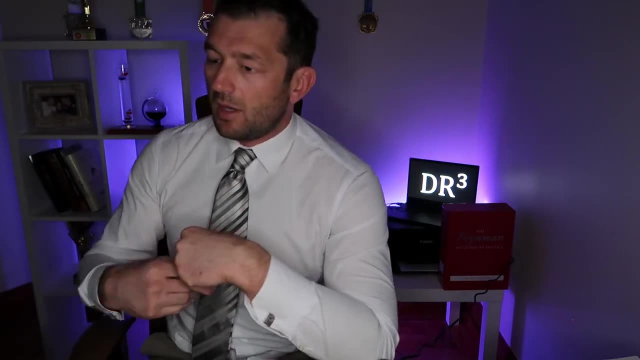 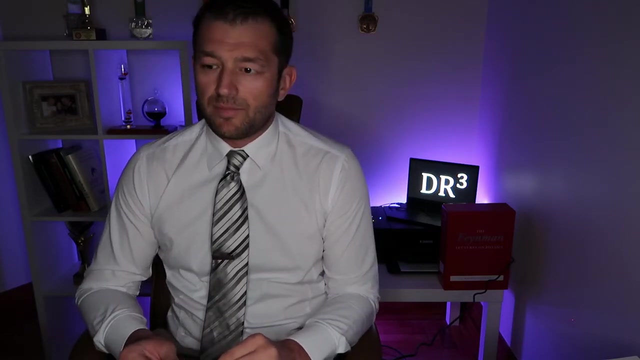 weather chart and the isobars are very close to each other. the pressure gradient is very strong, and then the pressure gradient force, consequently, is also very, very strong. Lastly, I promised you that we will also describe the process of breathing using the pressure gradient force, and this is really very, very 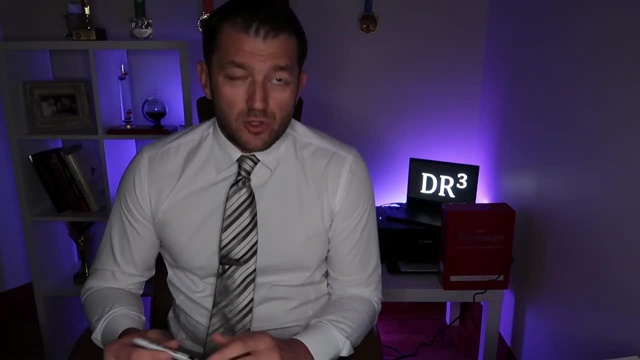 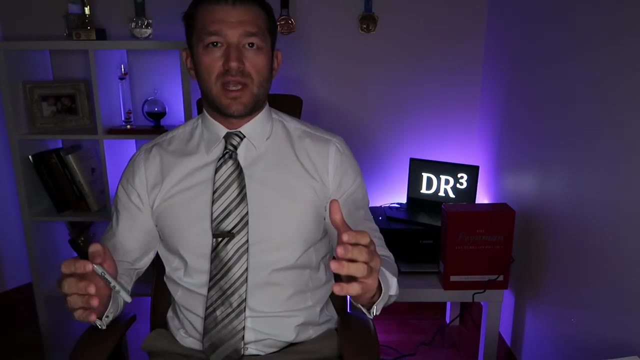 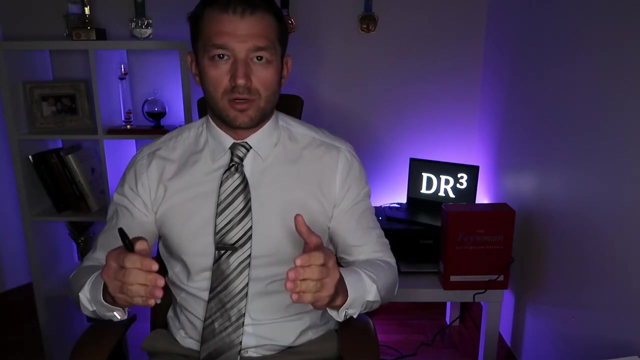 simple. You probably know from high school- if you don't know, you will learn in one of my future videos- that if you have a container of gas and you keep everything constant but you increase the volume of the container, then pressure consequently reduces and, as I said in the previous, 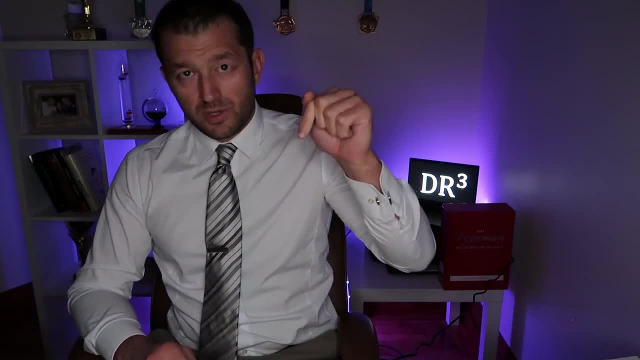 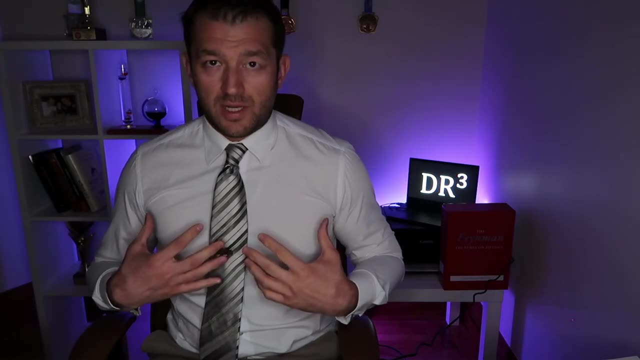 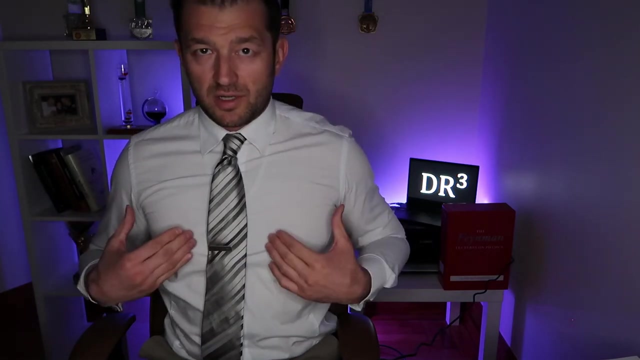 video on the continuum and I will put the link in the description so you can check out that video. our lungs are very good air container so when I breathe I expand my lungs. therefore the pressure decreases and there is the pressure difference between the air and the air. 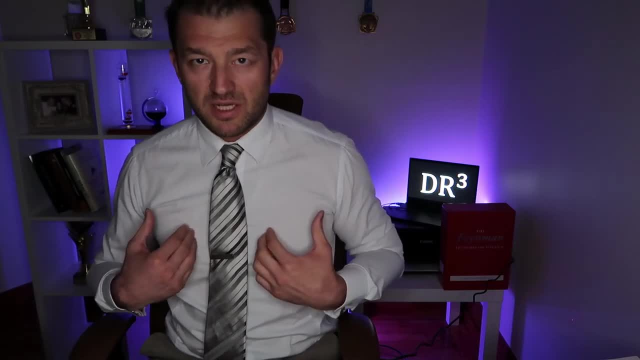 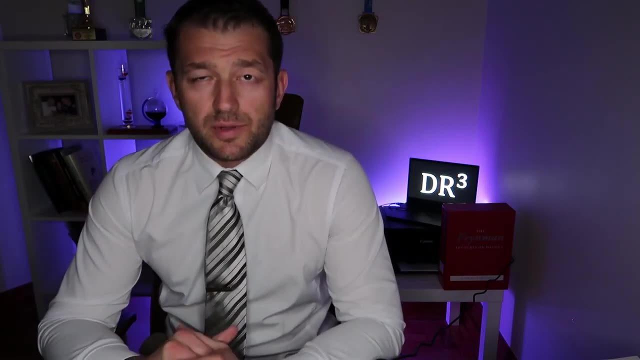 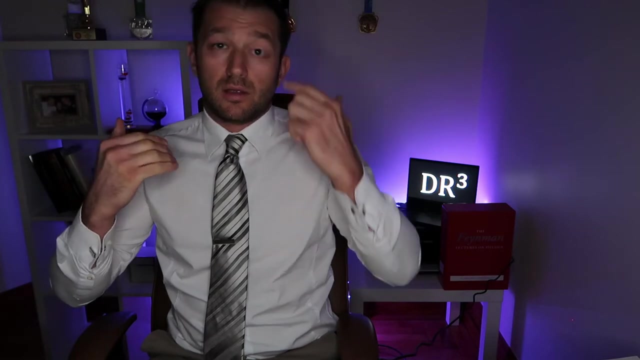 Pressure difference between inside of my chest or in my lungs and the atmosphere. if there is a pressure difference, there is the pressure gradient. if there is the pressure gradient, there is the pressure gradient force that is pushing air through my nose and the rest of the respiratory system to my lungs. Opposite happens when I contract lungs or my chest. the air goes out. so really the breathing has nothing to do with nose, except that air goes through the nose. if you would theoretically put the hole on your shoulder and somehow connected to your lungs, as you expand your lungs the pressure gradient force will force.